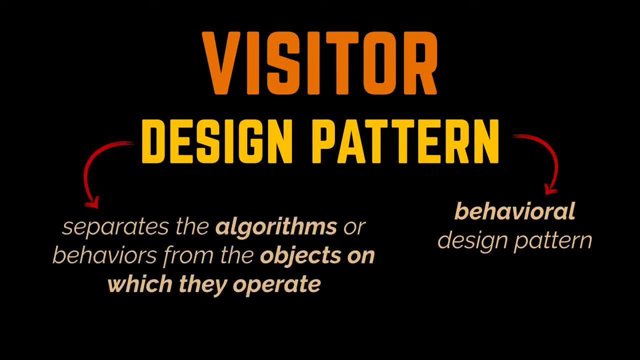 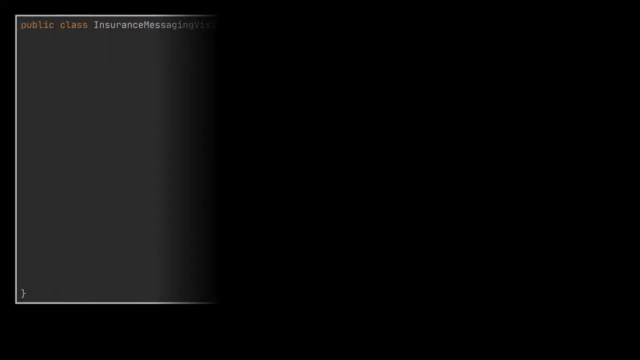 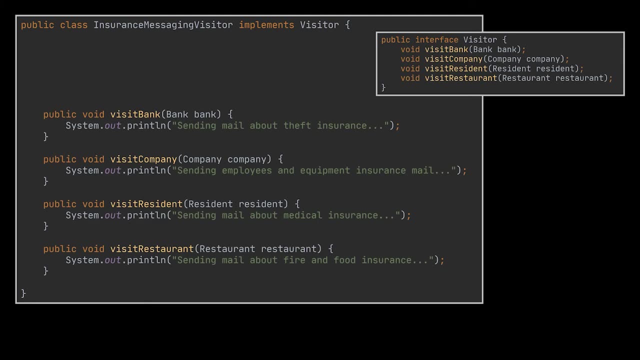 that lets you separate algorithms or behaviors from the objects on which they operate. let's try to apply it on our client's insurance example. to do that, I went ahead and created an insurance messaging visitor class alongside its visitor interface. then I moved all of our messaging behaviors to that particular interface and added their implementations in the corresponding 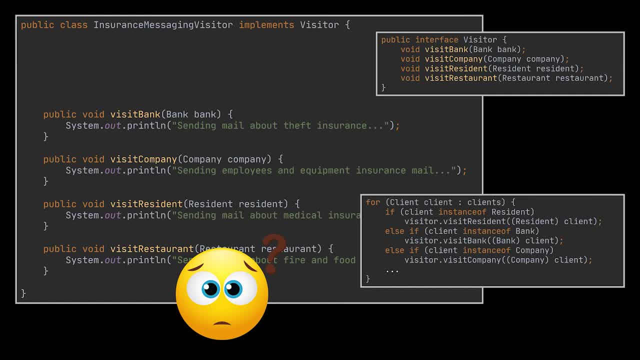 visitor class. but how exactly would we call these methods, especially when dealing with several clients? to pick the proper method, we need to check its class. doesn't this sound like a nightmare? you might also ask: why don't we use method overloading? go ahead and try to do that. your code won't even. 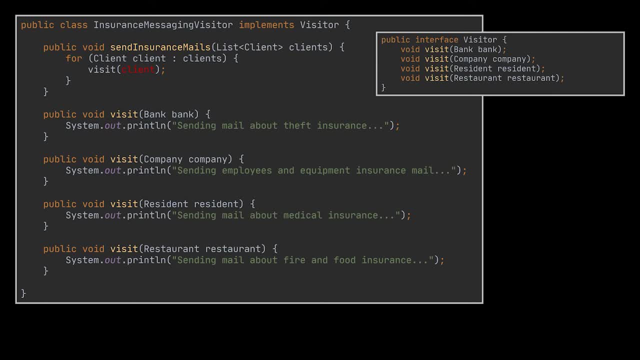 compile and will ask you to cast the client object to one of its sub classes. you see, the exact class of a client object is unknown in advance and hence the overloading mechanism won't be able to determine the correct method to execute. on the other hand, the visitor pattern addresses this by using a. 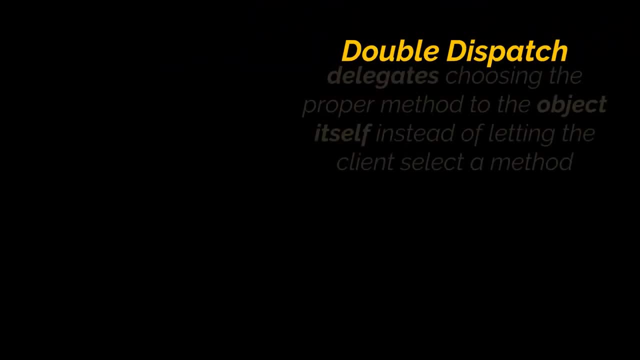 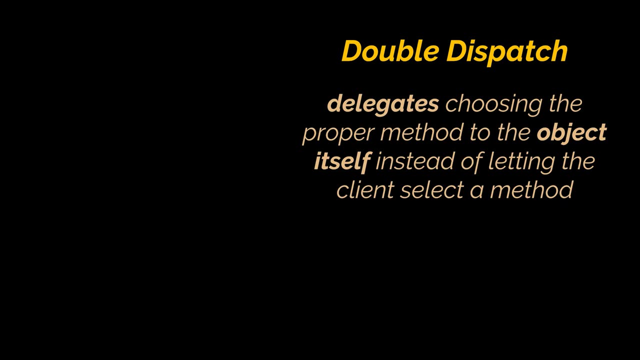 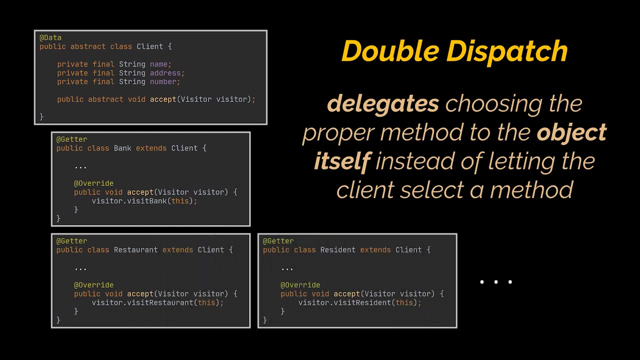 technique called double dispatch. since the objects know their own classes, the main idea here is to delegate choosing the proper method to the object itself, instead of letting the client select a method. so what each object will do is accept a visitor and tell it what visiting method should. 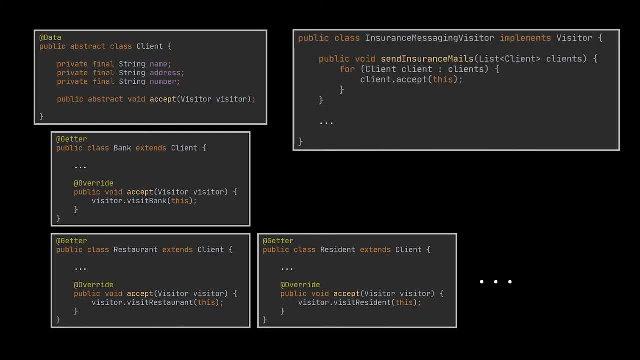 be executed and while dealing with a list of clients, all you have to do is invoke this method alongside a visitor. additionally, because we extracted all of these behaviors to a common interface, we can now easily introduce new visitors without altering existing ones. let's go ahead now and take a look at the structure or class diagram of the visitor. 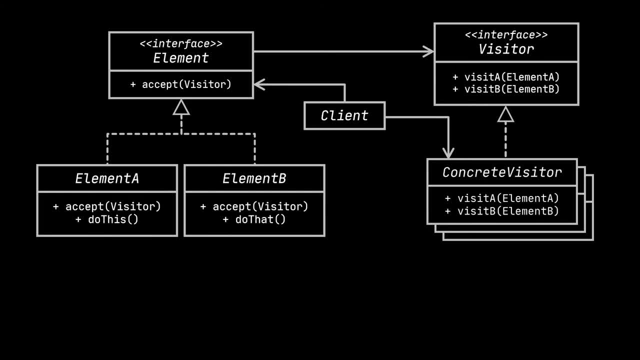 pattern while trying to relate it to the insurance example we just implemented. the first thing you will be able to relate to is the visitor interface. the interface declares a set of visiting methods that can take concrete elements of an object's as arguments. Next are the concrete visitors, which were represented by the insurance messaging. 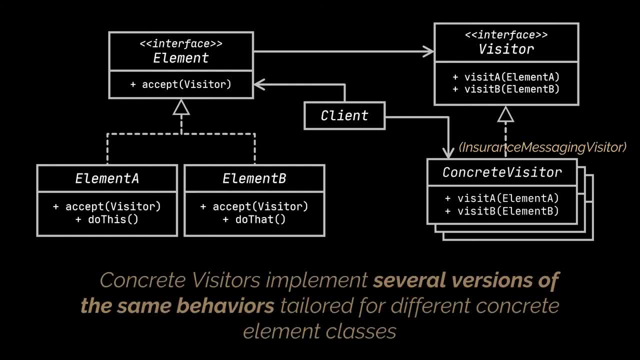 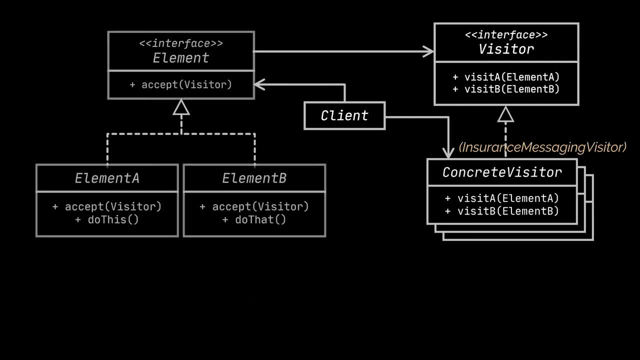 visitor class. in our example, These classes implement several versions of the same behaviors, tailored for different concrete element classes. Speaking of which, the concrete element classes and the element interface you see in the diagram were represented by the different types of clients and by the client abstract class respectively. in our insurance example, The element interface.